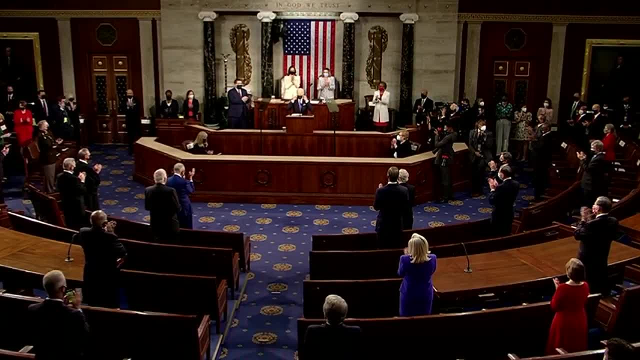 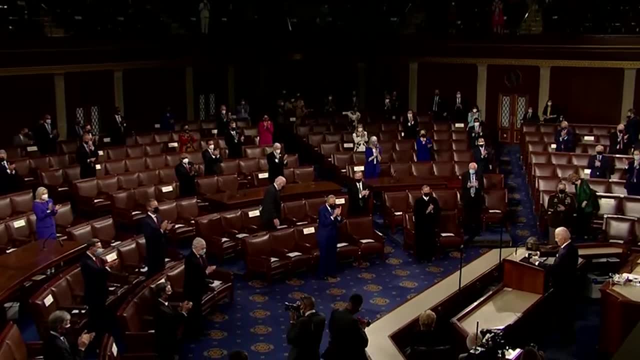 going through Congress before being sent back to the President to sign, And then the actual final dollar amounts can even vary somewhat from the enacted, But for our purposes these figures are close enough to get a basic idea- The easiest way to get a good idea of where the money goes. 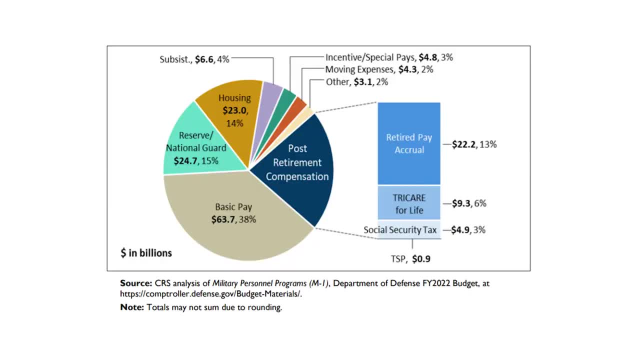 is breaking it down into categories: The military personnel budget and the budget for the US military. The US military personnel budget and the US military personnel budget, which includes base pay for personnel, retirement housing, etc. Which ends. 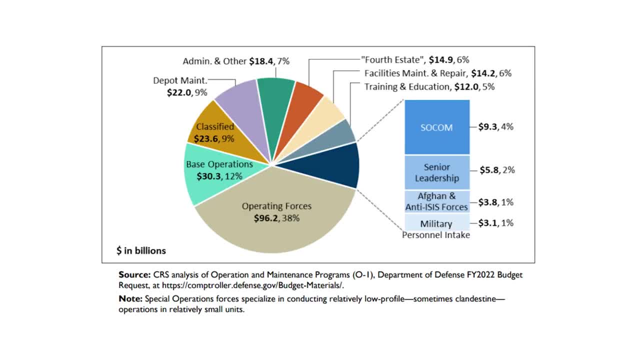 up accounting for 23% of the total budget. Operations and maintenance, which takes up the most, at 36%. This includes fuel supplies, spare parts, routine maintenance and major overhauls of aircraft, ships, ground vehicles, electronic support equipment and facilities, as well as 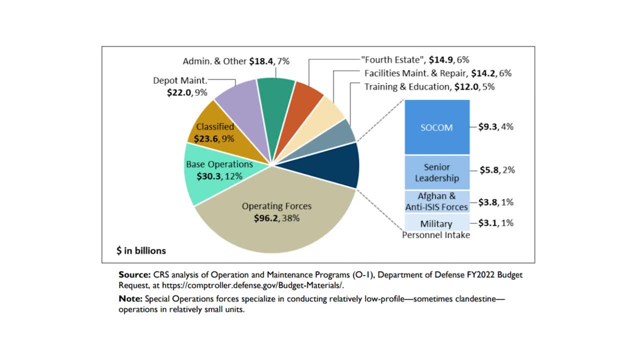 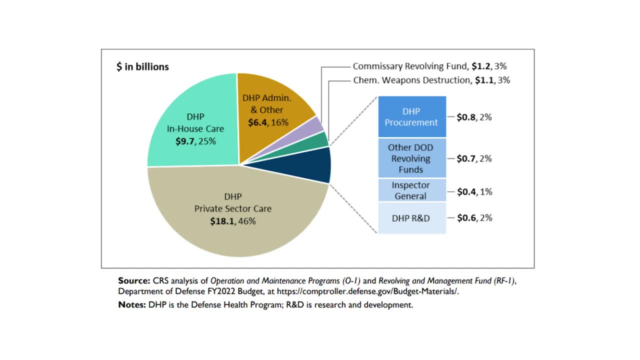 recruiting, training, education, administrative activities, headquarters and supply operations and much more. Then there's military construction at 1%, 5% to the health program, 19% on procurement, that's missiles, bombs, tanks, ships, aircraft, etc. 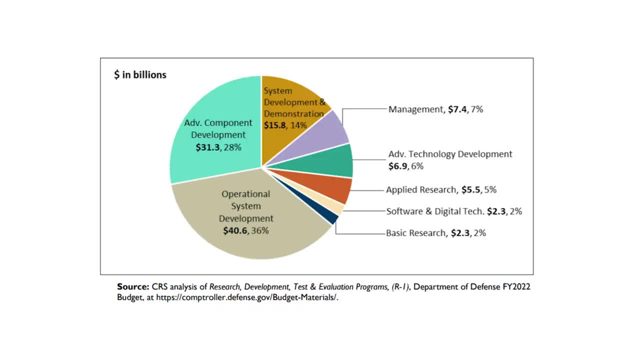 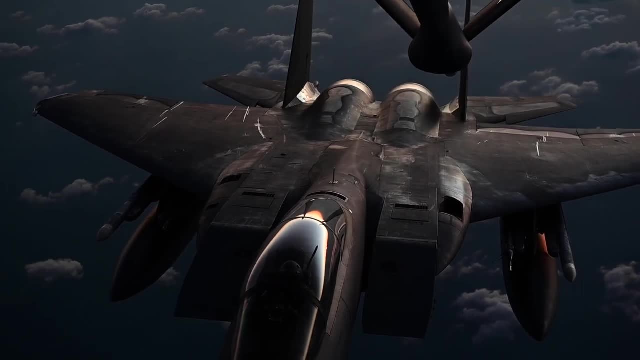 And finally research and development: the remaining 16%. That's the breakdown. Often, when people just mention flat out numbers or make statements like the US spends more than the next 11 combined, they're implying that the US is spending too much. 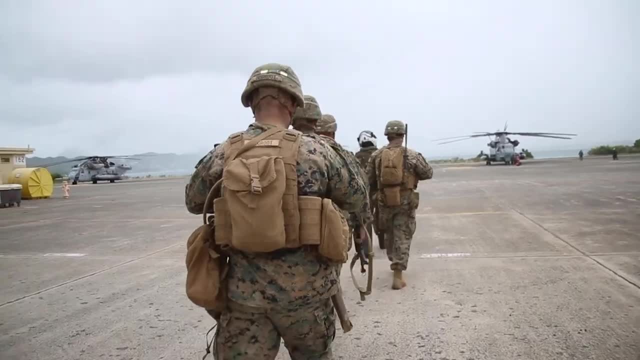 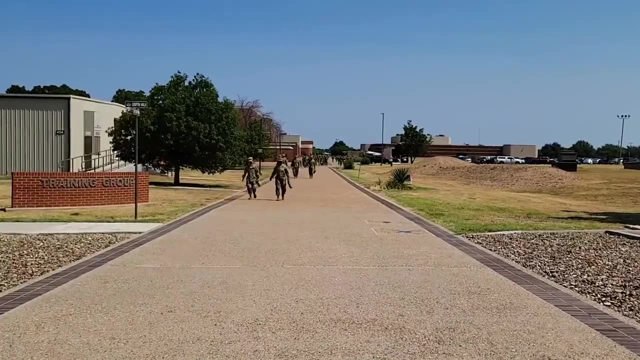 and it needs to be reduced. And maybe they are right, But any fruitful discussion requires more than that, like stating specifically where they would cut. Is that personnel wages, Or maintenance and operations, Or maybe research and development? And the same is true when people 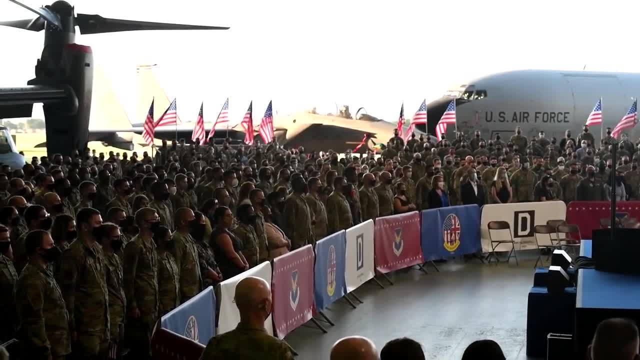 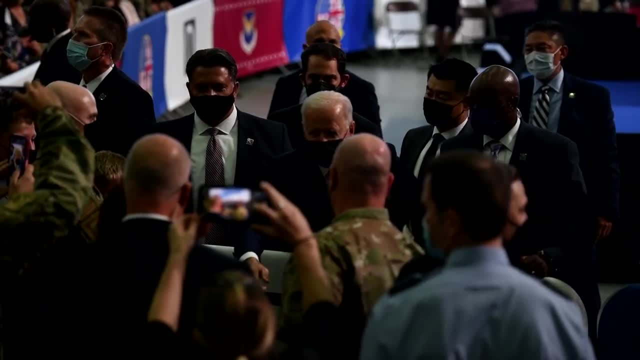 advocate for paying active military more. Maybe they are right, But with it already costing nearly a quarter of their entire budget, even small increases easily cost billions of dollars, So my point is vague. uninformed, blanket statements never lead to any efficient or 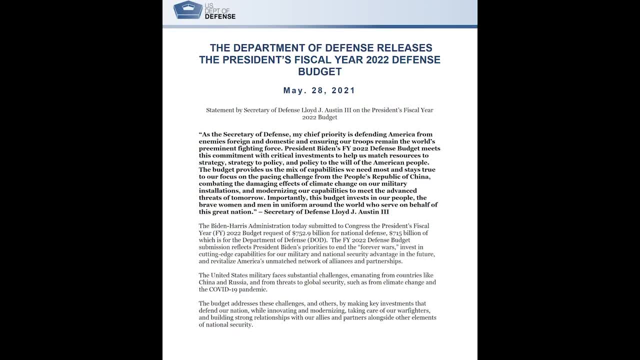 effective change. It's important to know the details. It's also fun to look up where the military is now and you'll see their faces in front of you. It's important to know the details. It's also fun to look up where the military is now and you'll see their faces in front of you. 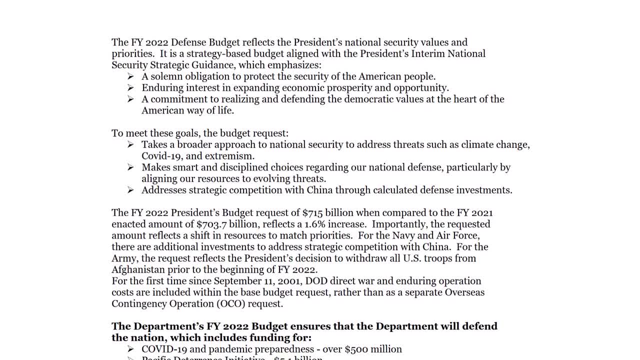 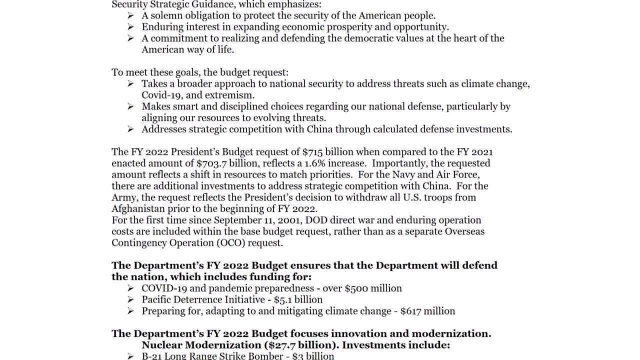 through the budget and read the way it's being presented. Every year it's presented as the most ingenious, effective budget that solves all defense problems for the US. The latest defense budget not only takes on Russia and China, but also climate change and the virus, But on a serious